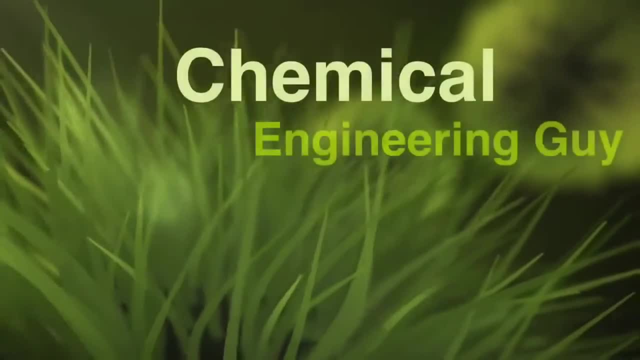 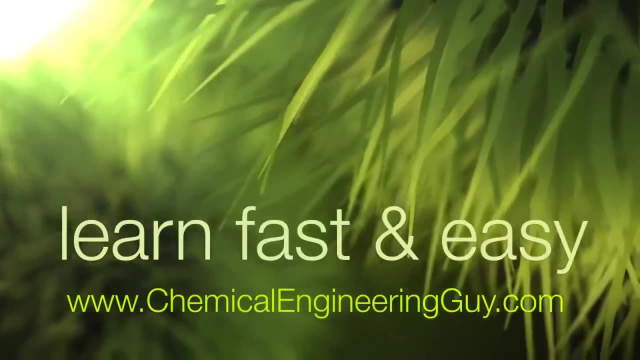 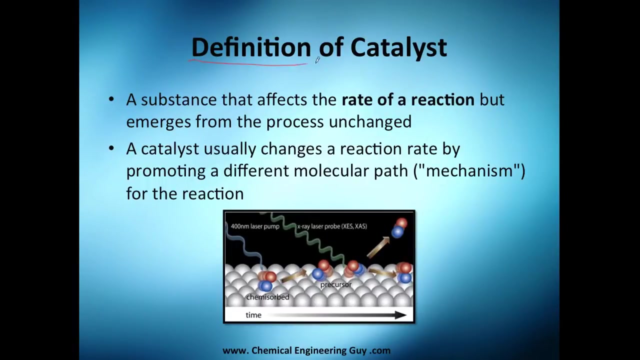 What's up, guys? let's start with the formal definition of what a catalyst is. and actually it's any substance that affects the rate of reaction, but it's not consumed and it's not changed and it's going to stay like that, even though you are experimenting. a rate of 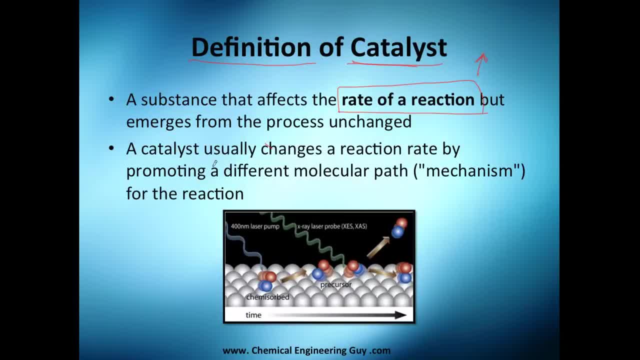 reaction normally higher than normal. The catalyst usually changes a reaction rate by promoting different molecular paths. we're going to see that later, but you know it. it's a mechanism, we've seen it before and essentially is: instead of going from a, let's say this is high energy, and you produce C, 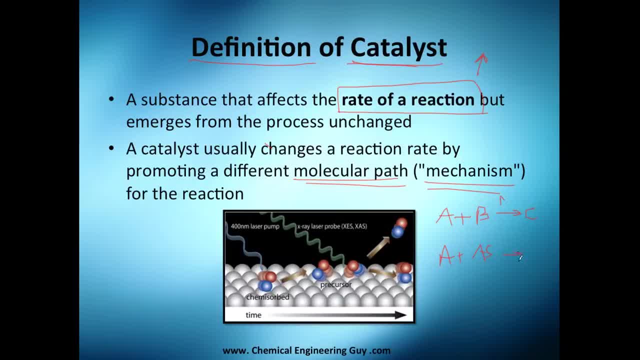 you're going to go and form As, and then As goes and forms S2, and then As2, gets B, and then AbS2 goes and forms S2C, which is C, and then it dissolves and you produce. 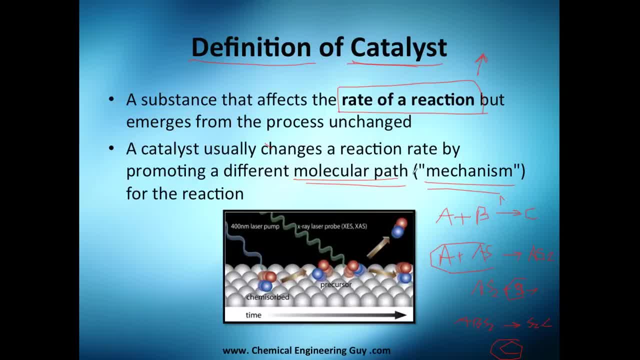 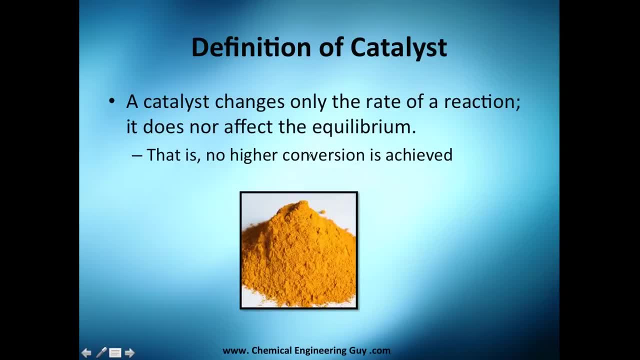 eventually, from A and B, you're going to produce C, So essentially, you have different paths in which they will require less energy and, of course, will go faster. because of that, It's very important to tell you guys that it only changes the rate of reaction, that 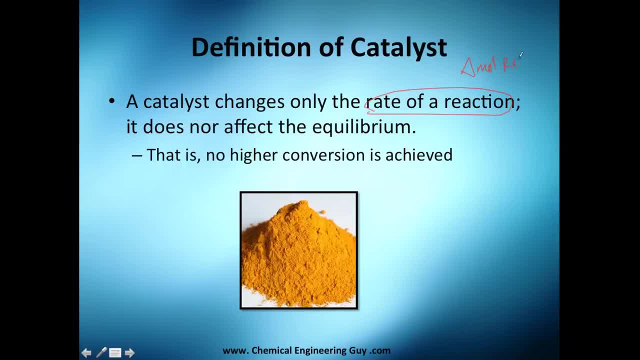 is how much or how many moles are reacting per unit time, but does not affect the equilibrium. that's more into thermodynamics. we're going to speak right now only, but only on, with kinetics guys. So equilibrium is not going to be changed. for example, you know, A plus B produces C. 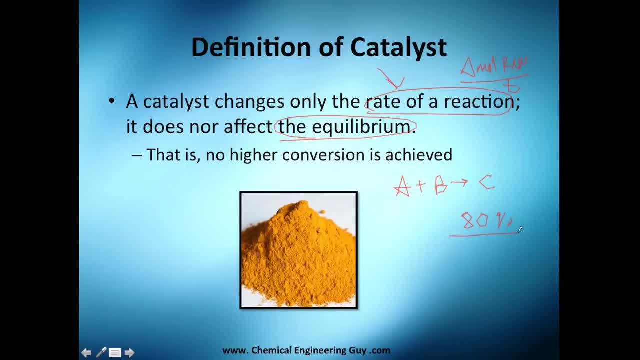 and you know that, abnormally, at this rate Temperature, you will only get 80% and let's say 5 hours. well, we're going to see that that will be the case as well, but, for example, the same percentage is going to be achieving. 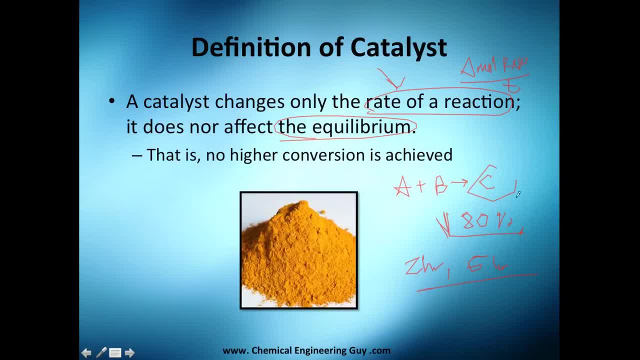 2 hours, let's say so. You're going to have C, also 80%, So no higher conversion is achieved, even though we're going to find later that certain catalysts, for example, you have A and B and you add them palladium, you will react C. 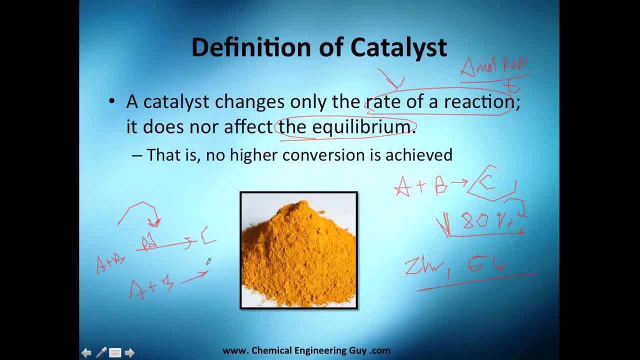 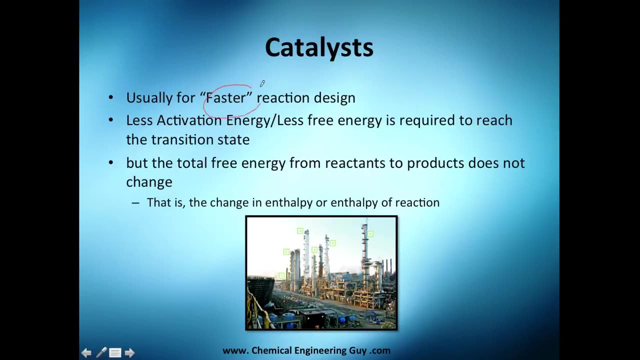 but if you were to have only C, A and B and no catalyst, you will react. anything so technically you will not react. so what you want is, of course, produce that. Let's continue a little bit on catalysts. they usually go faster for our reactor design. 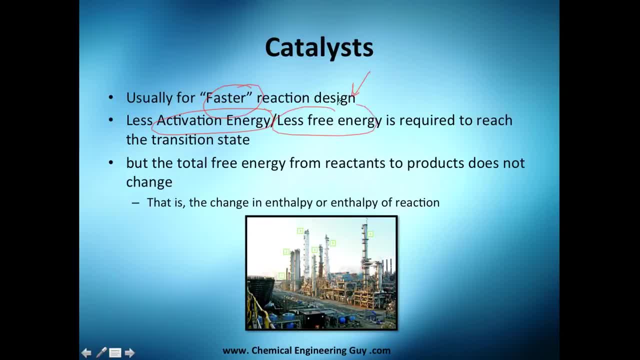 it requires less activation energy and less free energy to reach the transition state. and you know the transition state. we're going to see that later. But essentially the energy required to get into A and B ready to react is going to be decreased. Also, the total energy guys on the molecules will eventually not change the enthalpy of 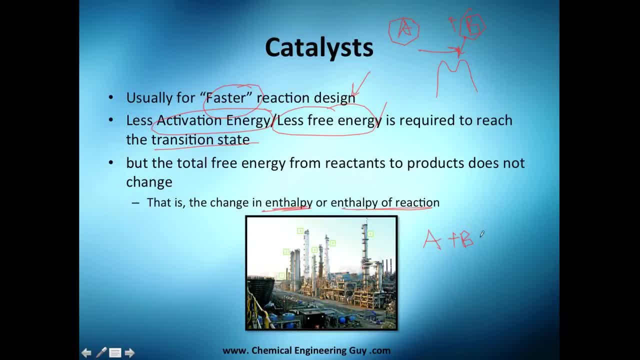 reaction is not going to change. You need A plus B to react C and you have a delta of enthalpy. And if you use a catalyst, Even though it's going to be faster, you still you're going to have the same change. 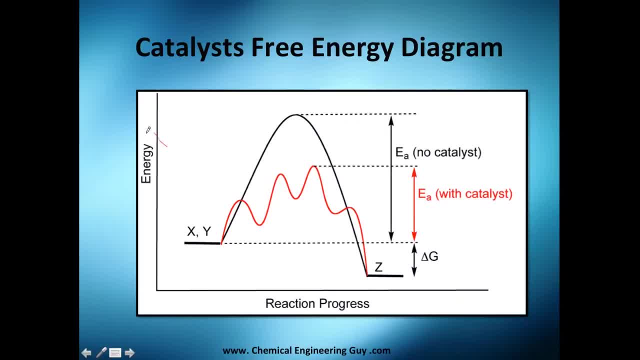 on enthalpy. that's very important, guys. Once again, let me show you the energy. this is about free energy. you don't think it's about enthalpy. So you know X, Y and C is our product. 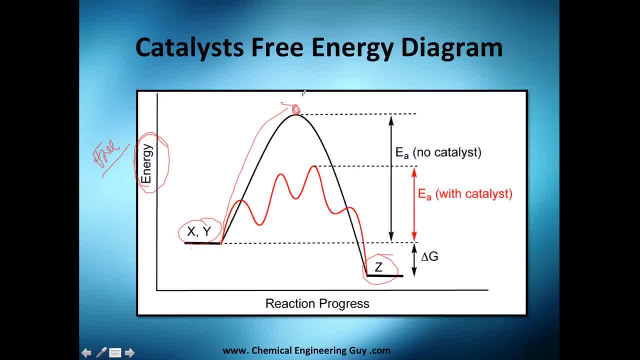 They will need to experience high energy. they will need to collide and crash between them in order to start reacting. Once they start reacting, you start liberating energy, And this is the energy I'm telling you about: the activation energy plus the free energy. 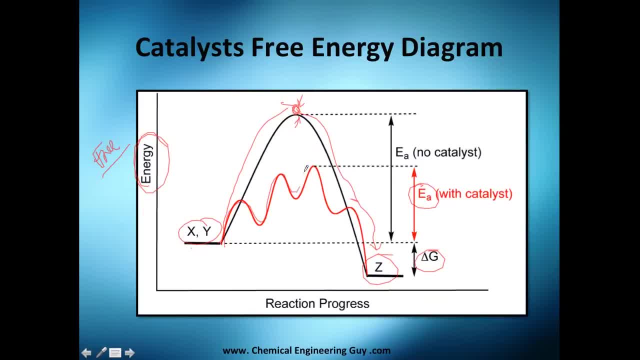 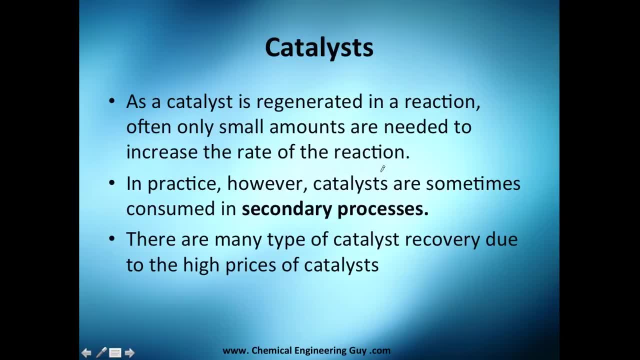 And if you were to add a catalyst, you're going to need less energy. Look, maximum energy is going to be almost half of that original. Normally, if you had a perfect case, you will never need to get more catalysts, but the 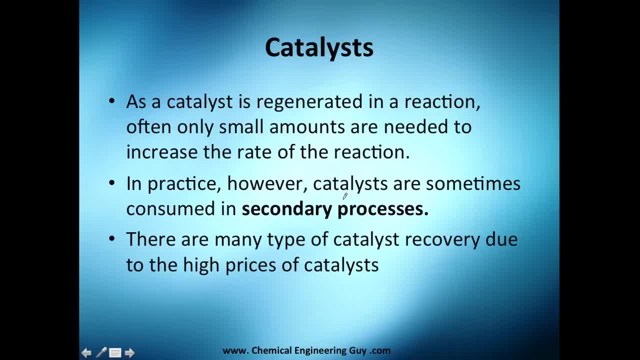 actual case is that catalysts will either deactivate, they will get poisoned, they will die, They will get coked and they will be reacted in secondary processes. So you go and you will need eventually to recover that catalyst material. There are many types of catalyst recovery due to the high prices of it.